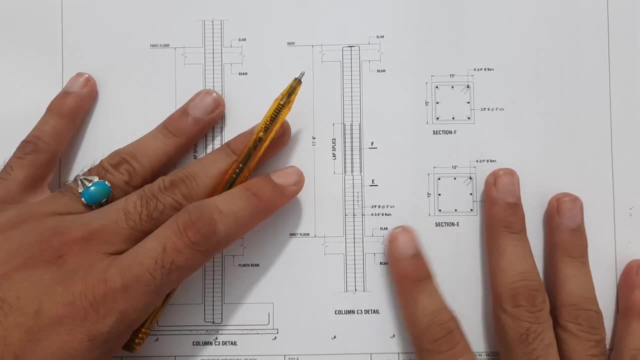 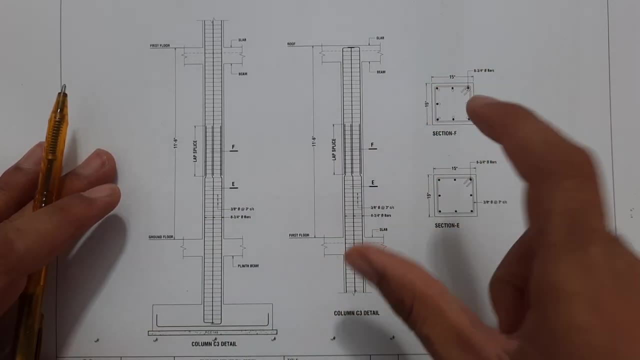 Assalamu alaikum guys, welcome back to civil engineers YouTube channel. today I will guide you how to read column drawing on construction site, specially at steel structural design, if you are working on construction site. so you should have watched this video till the end to learn. 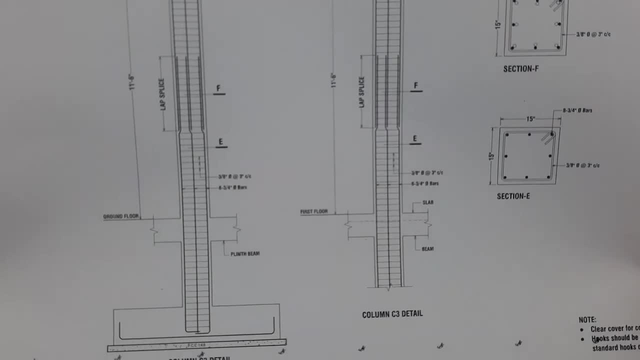 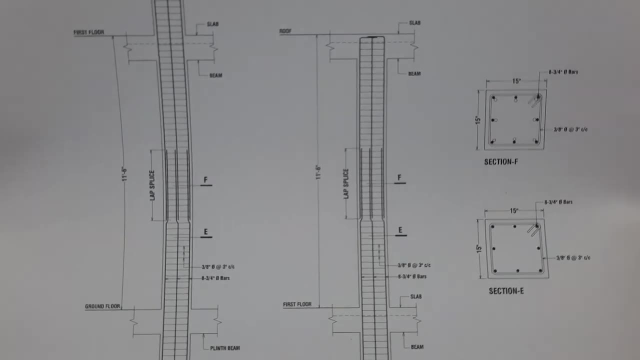 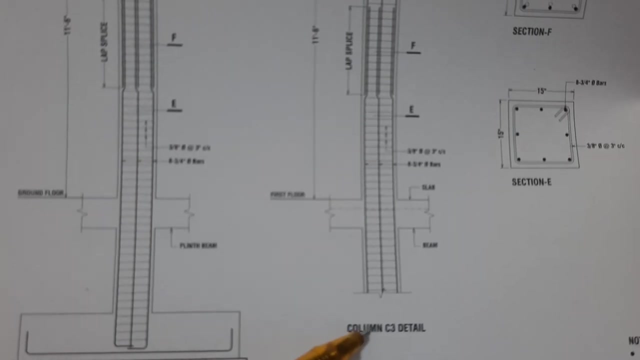 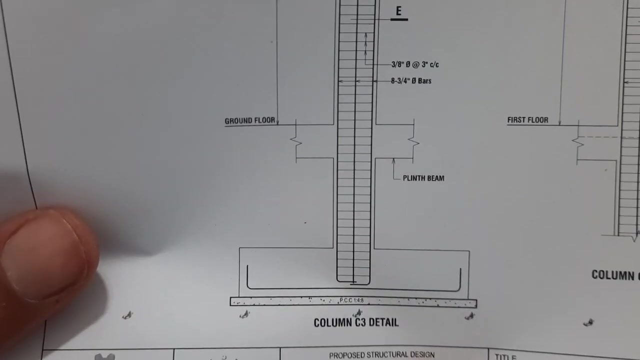 something new: how to read structural drawing for column column details on site. so let's get start, guys, if this video is helpful for you, so you may like this video. guys, here you can see this is column c3 detail. this one- okay, let me focus the camera right- and the next one is column c3 detail. 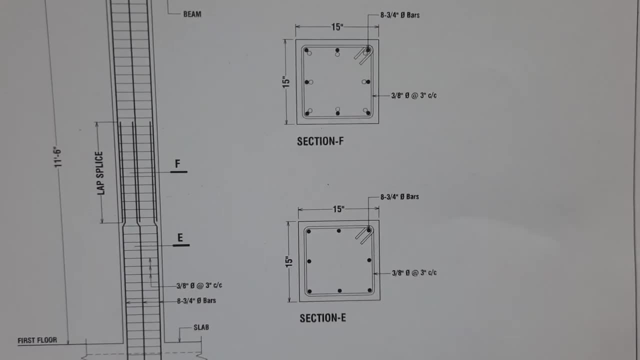 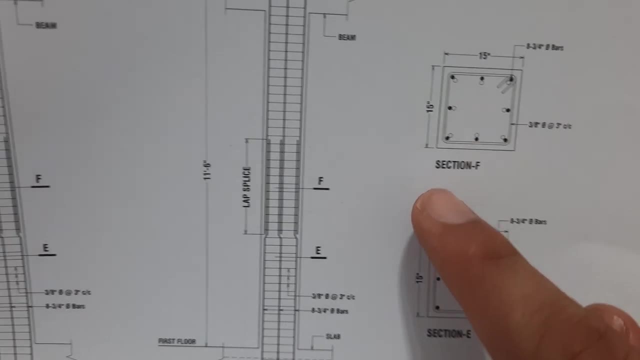 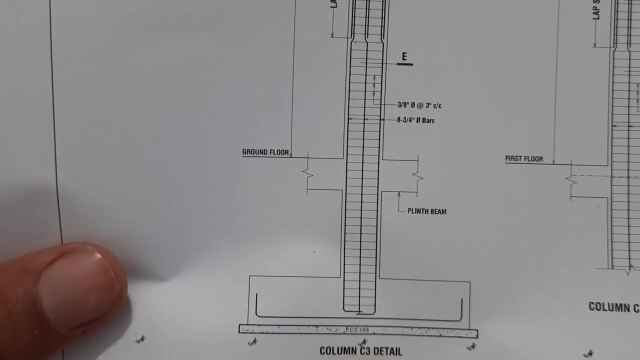 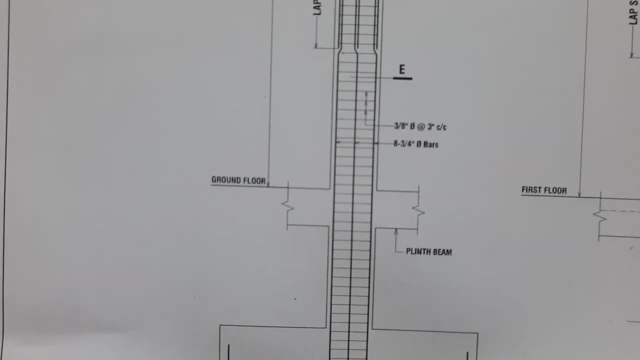 also. okay, you can see, guys, here the sections. we have two sections section, section E and section F. okay, for this column we can use these two sections, guys, if you, if you see at the bottom, so they used here it means pcc, one for air ratio. okay, but they didn't mention the dimension. so 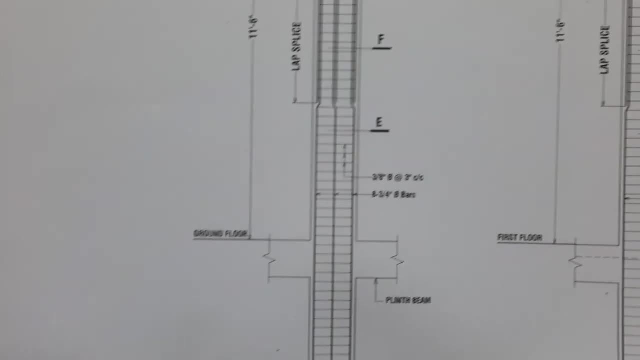 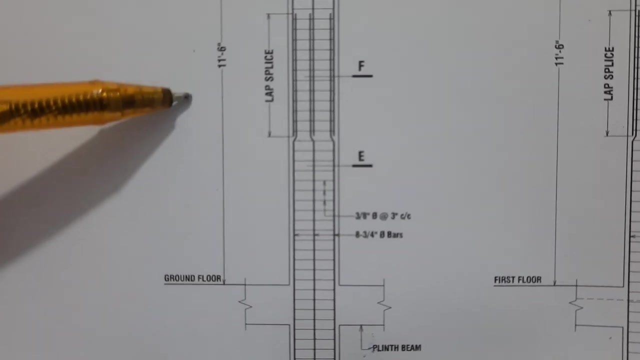 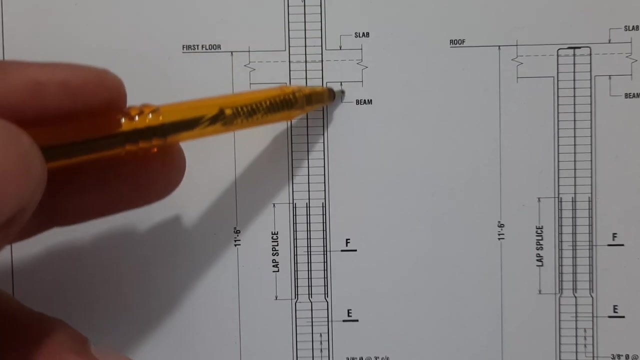 therefore ignore this now. just I'm telling you how to read. but here and the footing: you can see this is the plant beam if you see it's ground floor. so the ground floor height is 11 feet 6 inch. right here, guys, you can see this is beam and this is slip. okay, as you can see the dotted lines can. 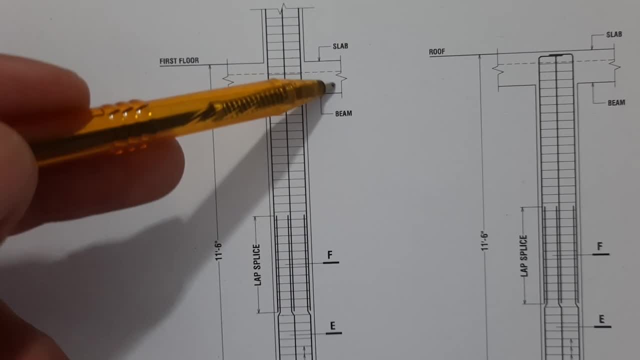 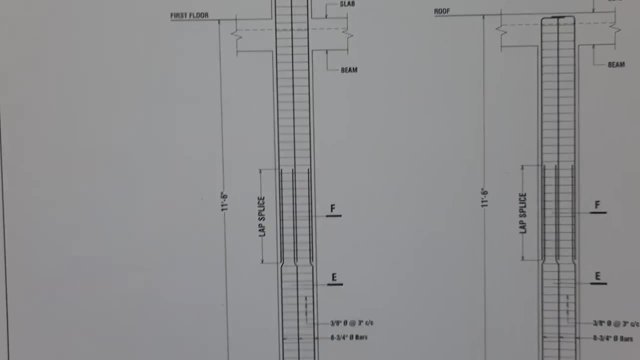 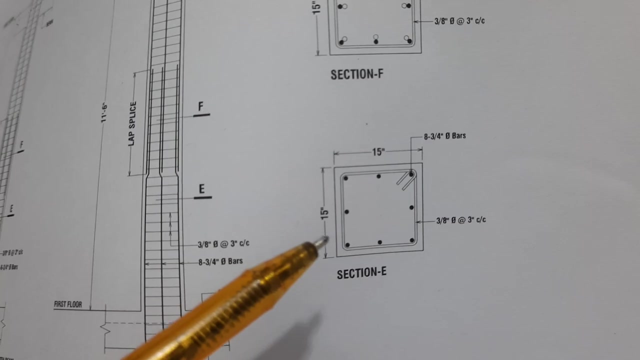 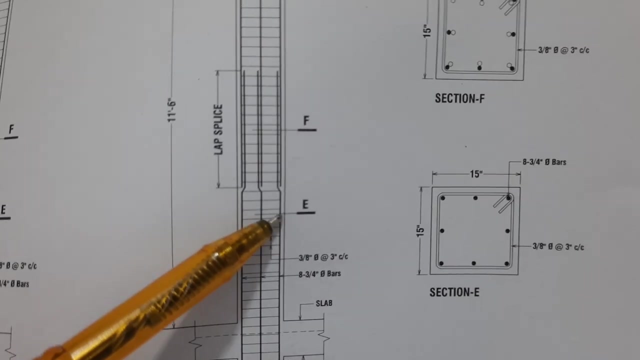 be 6 inches and the beam is at the bottom. okay, on the top of the beam we have a slip. this is first floor. now you can see here clearly. now, guys, here, let me discuss its section here. guys, you can see section e. so here, if you see this point, this is section e, so section e can show you we have here. 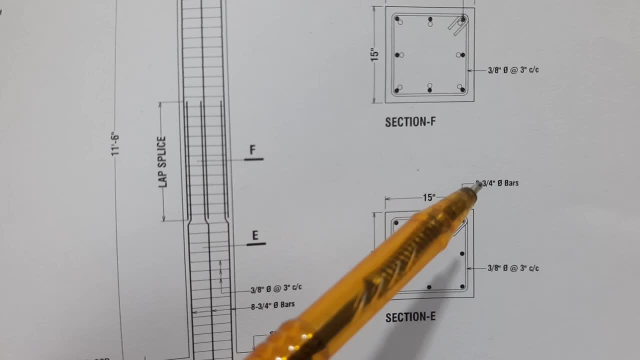 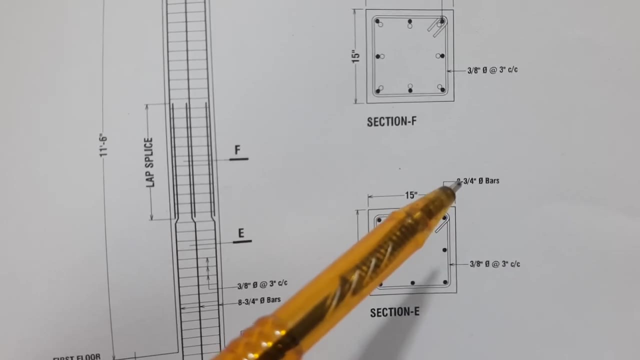 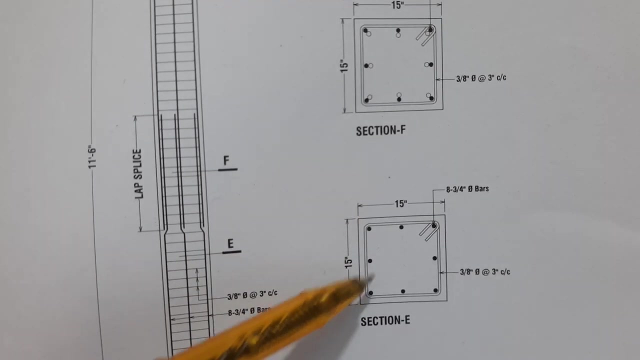 8 steel rods, SEAT rats on the septal side. seven, eight steel rods, 8 steel rods which dyea is three by eight. three by four means six Dahye of Steel rod. right size of this size of the column is, with concrete, 15 by 15 inches and you can see the hooks which are built with 135 degree if you see its.